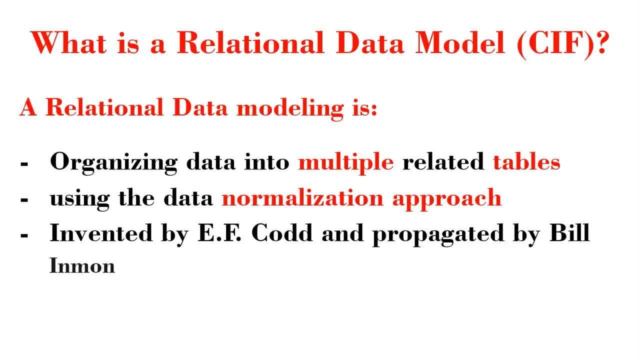 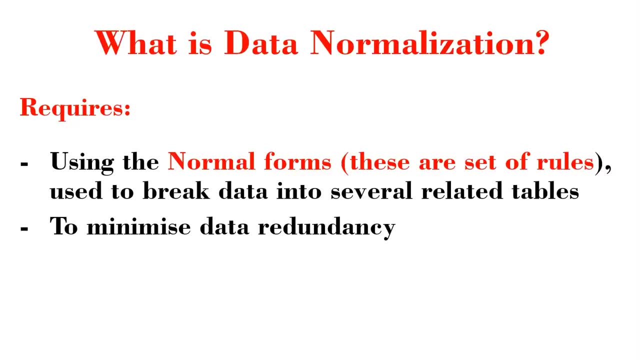 was invented by EF Codd and propagated by Bill Aylman. So you would ask: what is data normalization? Well, it's the use of set of rules to break a chunk of data into multiple related tables, and the purpose of that is to minimize data redundancy. 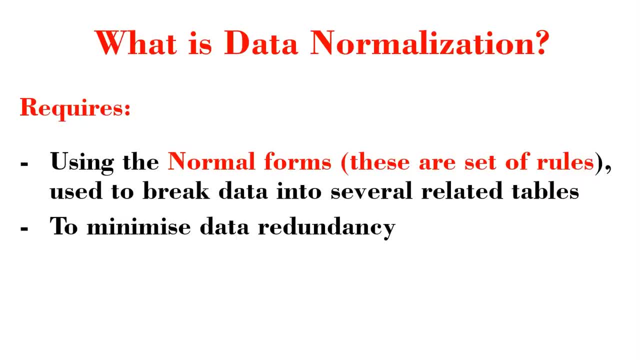 Although there are several data normalization rules, in this tutorial we are going to discuss the first three normal forms, Or the first three normalization rules, And if you are able to effectively apply these first three set of rules in your relational model, your data will be well normalized and, trust me, 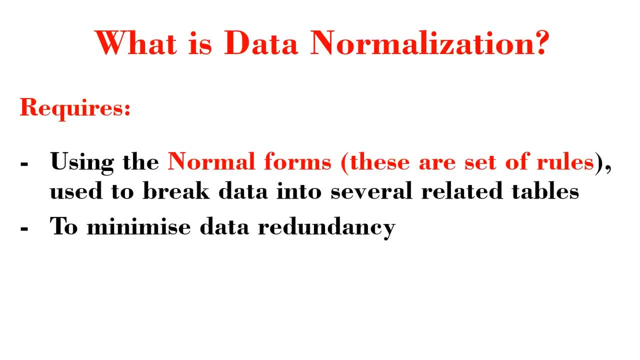 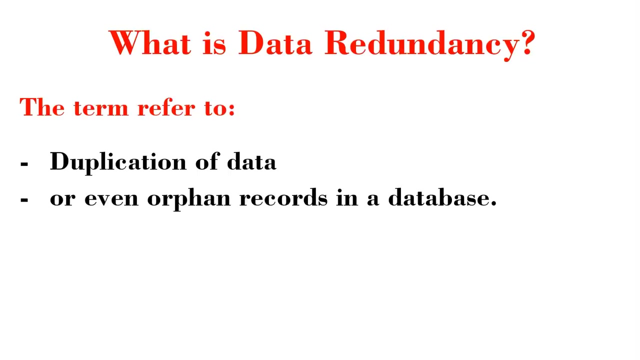 you won't be needing any other subsequent type of normal forms, But for your knowledge, you can read further about the other normal forms. I mentioned that we normalize data to minimize data redundancy. So what is data normalization? Data normalization is a term used to refer to duplication of data within a database, or even 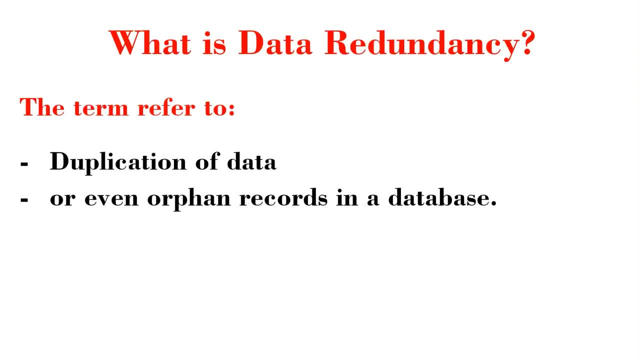 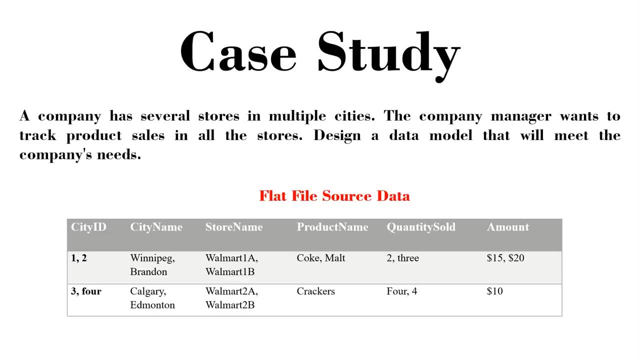 orphan records present in a database, And you would see this as we move along in this tutorial. As I've mentioned previously, our explanation of data normalization today is going to be based on this case study and I've provided a copy of the case study below this video in the description. 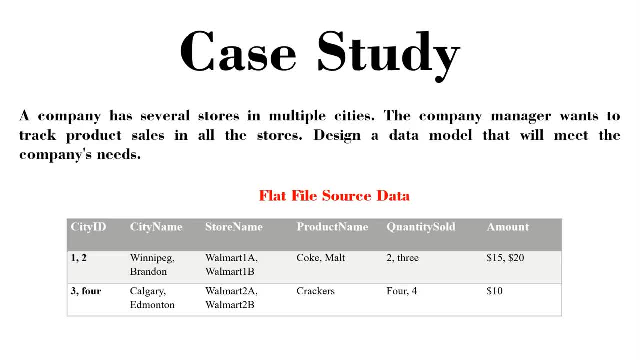 so feel free to refer to it as you follow along. And in this case study we have a company that has several stores in multiple cities. The company manager wants us to track product sales in all the stores and design a data model that would meet the company's needs. 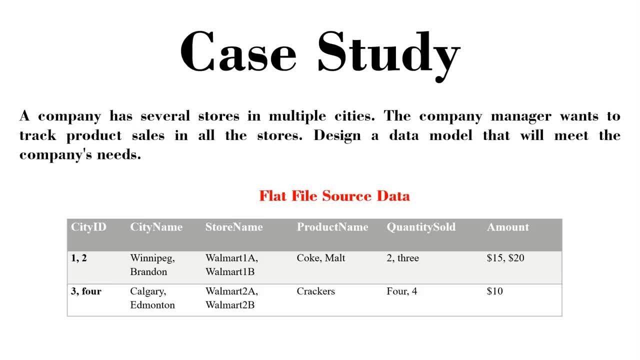 He also provided us with source data and this is the data that he gave to us as data modelers to use to help him solve his problem In relational data modeling. this table is unacceptable. At first glance, we can easily see that even this table violates the first normalization rule, or the first 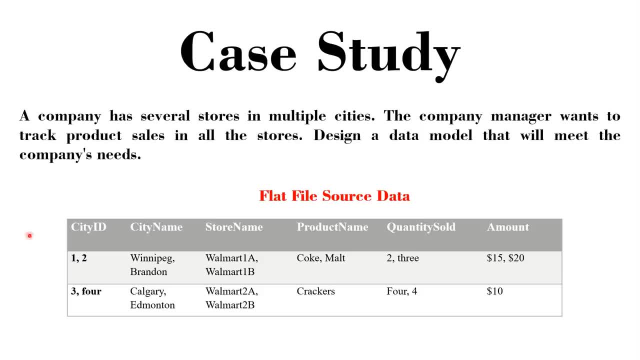 normal form, because we have more than one values in some of the columns separated by comma, and also we have different data types, because we have two. We have two types of data types. We have three types. within a particular column, For instance, we have this three value, which is an integer. 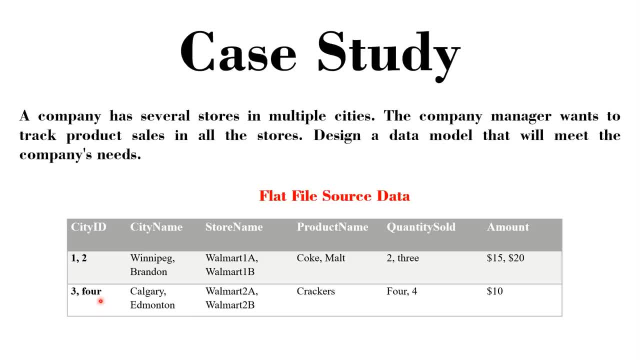 and then we also have four, which is a text data type. We cannot miss data types within a particular column. We have to stick to one data type. So we need to resolve this table and the first step is to normalize this table to the first normal form. 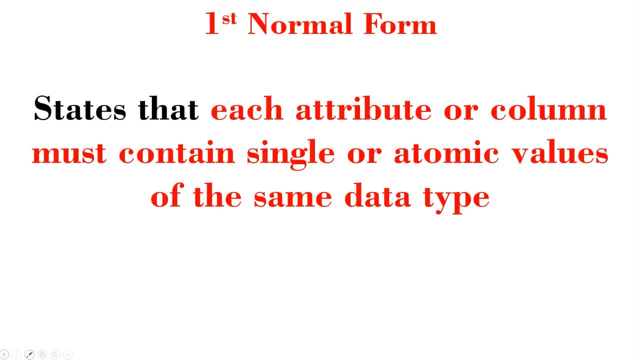 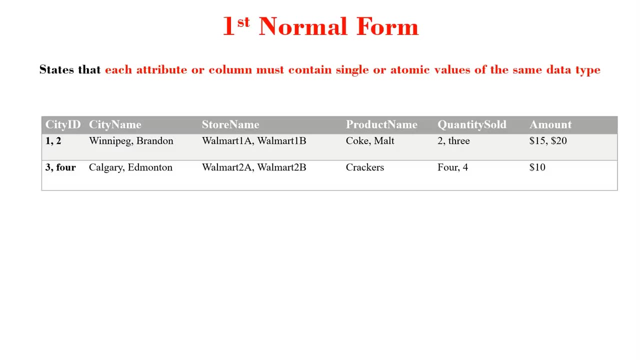 The first normalization rule states that each attribute must contain a single value and each value within a particular column must be of the same data type. What do I mean by that? Taking this table that the manager gave to us in order for us to certify the first? 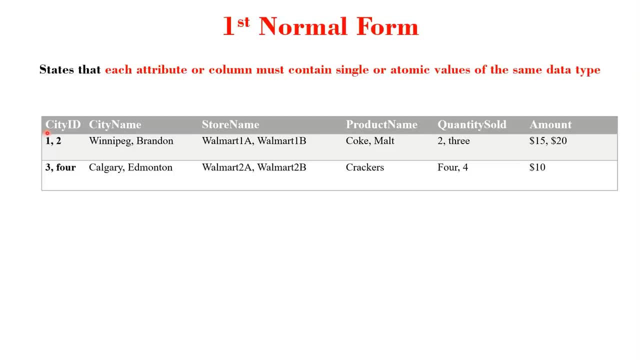 normal form, each column. for instance, taking the city IUD column, each column has to contain a single column. So, taking the city IUD column, each column has to contain a single column, single value. so we cannot have one and two all in the same row. we have to take 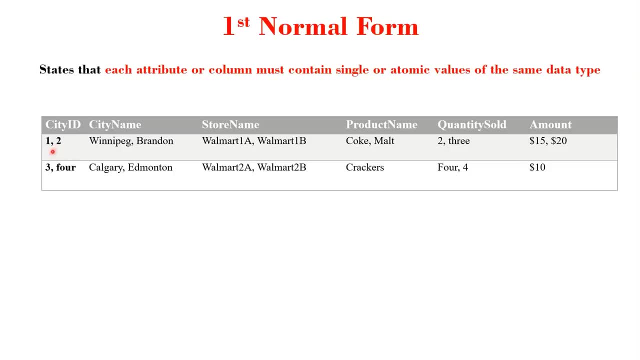 one of those values to the next row. so we have to take two to the next row and do the same for three and four. so in this table we supposed to get four rows. so at the end of the day for this original table to satisfy the first. 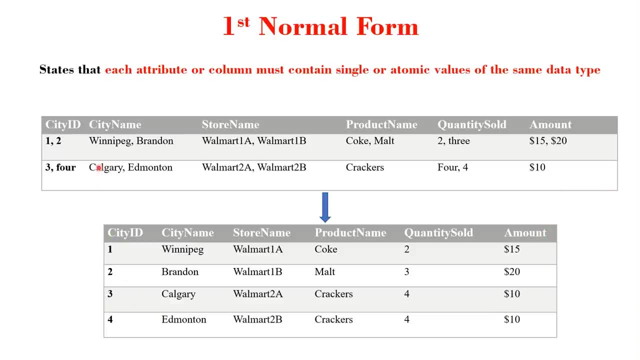 normal form. this is how it's supposed to look like. the first column, which is the city ID, has one, two, three, four values, so we break them down to four rows and then we move on to the city name: Winnipeg- Brandon. as you can see, it looks as if 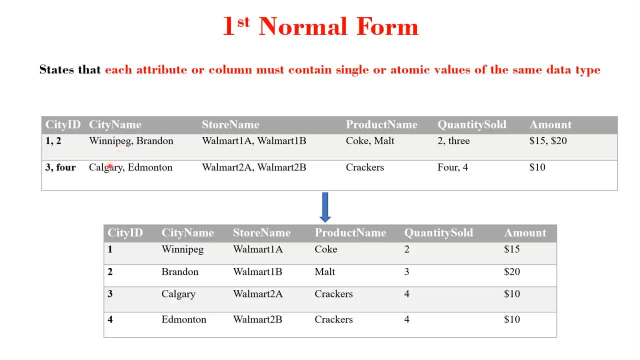 the one represents Winnipeg and two represents Brandon, so we have broken down for the city name. ideally, you need to talk to the business to find out if that is really how they intended to capture this data. but, looking at it is supposed to be broken down this way, one thing that I also want to emphasize on. 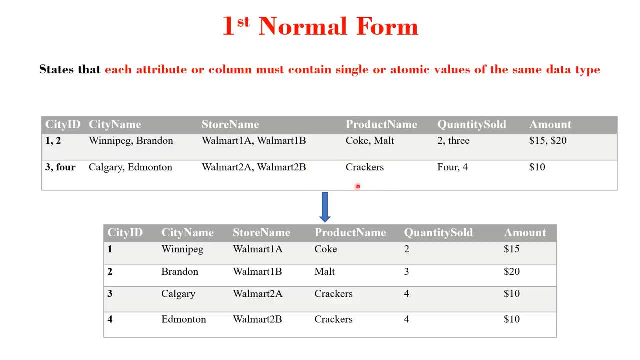 is this product name? you can see that we have only one product name. however, we have two city names, city IDs and store name, which tells me that this particular product name, which is crackers, was purchased two times. but because it's the same product name, they decided to just. 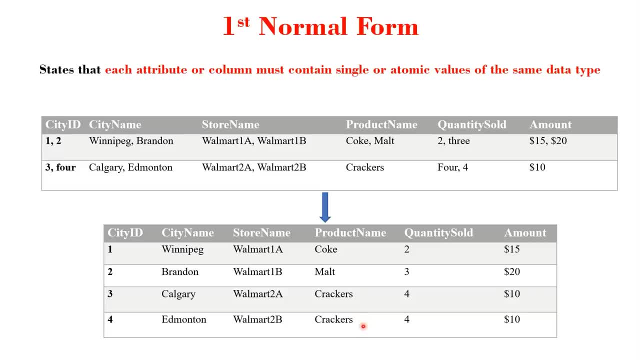 write it once. so I have represented it here two times. so in Calgary crackers was bought and also in Edmonton crackers was sold. okay, again, you need to talk to the business just to confirm that this is what they actually intended to do and you verify the product name as well. so yeah, with the WOW button we click this. 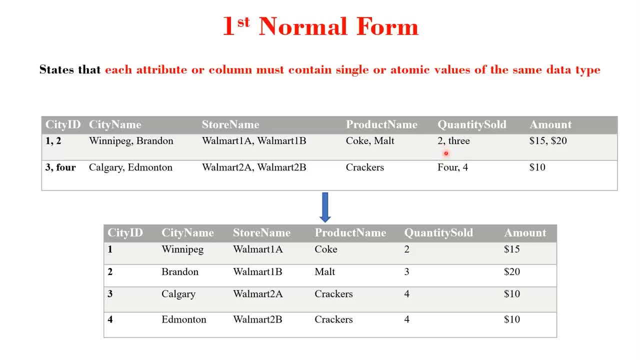 box. let's see, we can see this theowing method. this is the simple method, which곡, and we can see what the new works is, and so we want to consist it here. we want to continue testing this product action, so I'm showing some connaignances about it and this is how you can test the product, and I'm also going 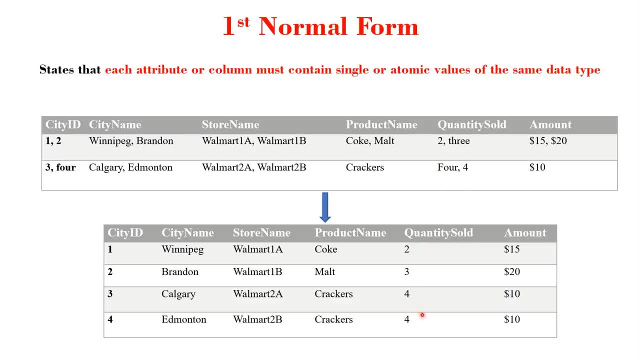 to talk about volumagnus in other resources as well. in order for you to next row, we have 4 and 4.. I've also done the same thing for the amount column. Okay. so what we have done now is we have separated the data in this table into. 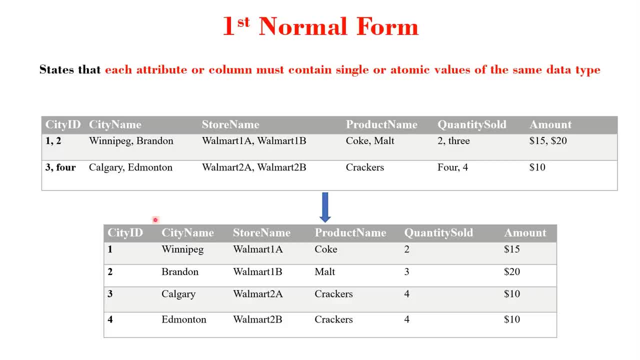 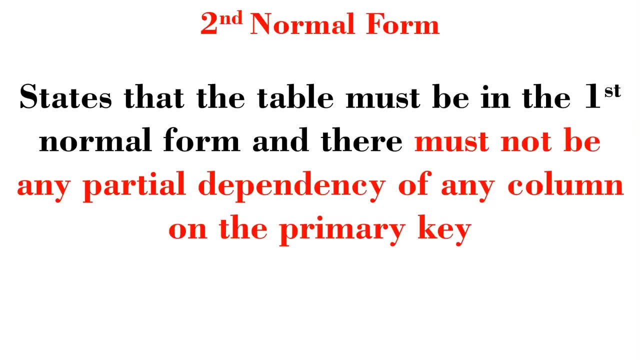 multiple rows and this table satisfies the first normal form. Moving on to the second normal form, the rule states that the table must first be in the first normal form and there must not be any partial dependency of any column on the primary key. What does that mean? Let's take our first normalized form table and 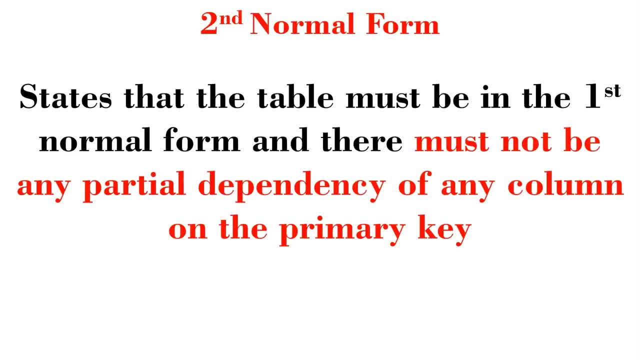 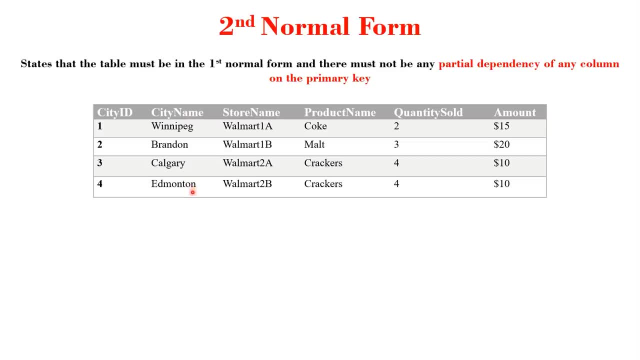 see how we can conform it to the second normalization rule. Here we have city name, which fully depends on the city ID. The city ID is a unique identifier of the table or the primary key. So city name fully depends on city ID. but we cannot say the same for the rest. 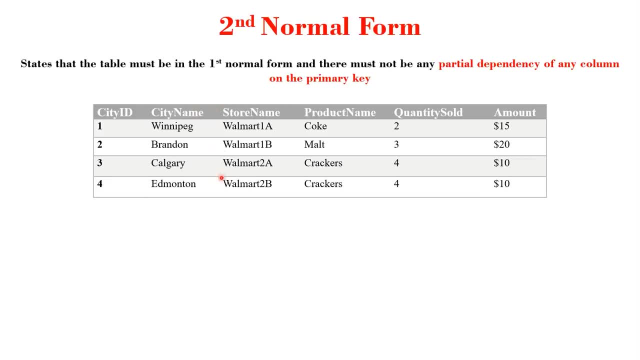 of these columns. So in the second normal form there shouldn't be any partial dependency of any column on the primary keys. These columns are not even dependent on the primary key, which is the city ID. So for this table to satisfy the second normal form, we have to move these columns that do not depend on the 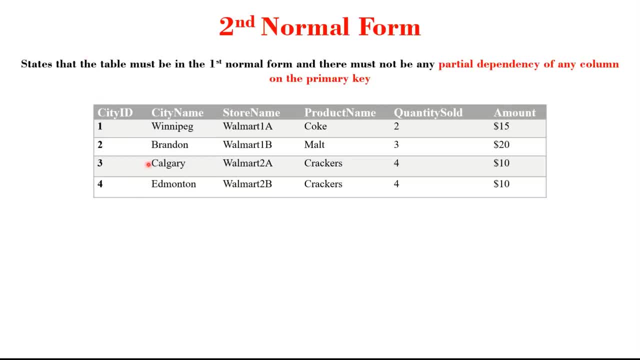 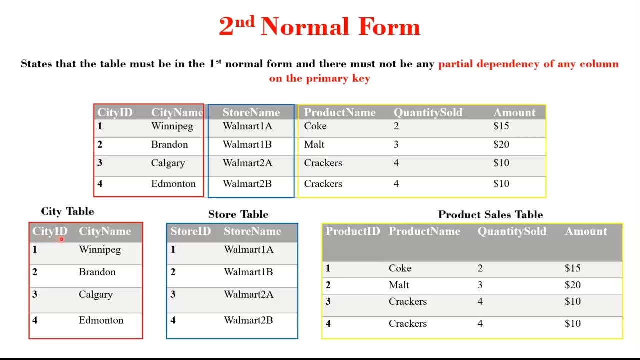 primary key into separate tables. So, for instance, we are going to have to create table for city name store and also for product, just as this, and each table will have its own unique identifier or primary key. So, for instance, in this city table we have city name as the column and it depends on the primary key, which. 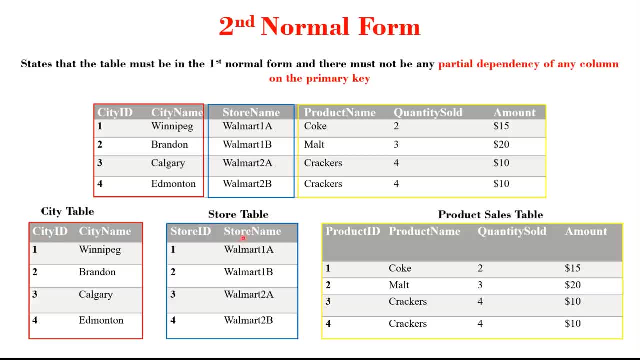 is the city ID. We also have a store table which is uniquely identified by this store ID and also we have product sales table and the primary key is the product ID. Product name fully depends on the product ID. These two columns- quantity sold and amount- are depending on the 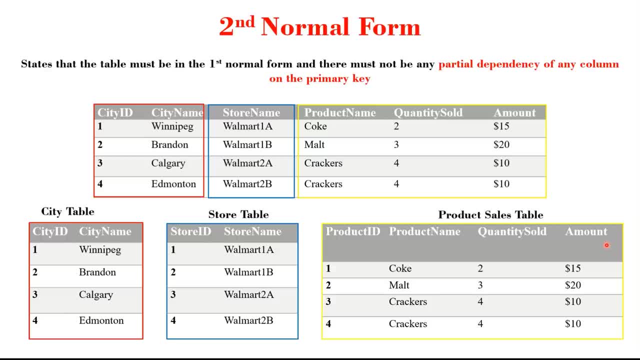 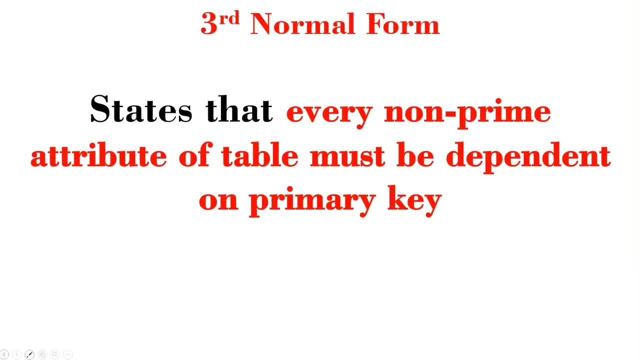 product name, and we are going to resolve this particular issue under the third normal form. So let's move on to the third normal form. For the third normal form, the table has to satisfy the second normal form and also every non-prime attribute of the table must be dependent on the primary key. 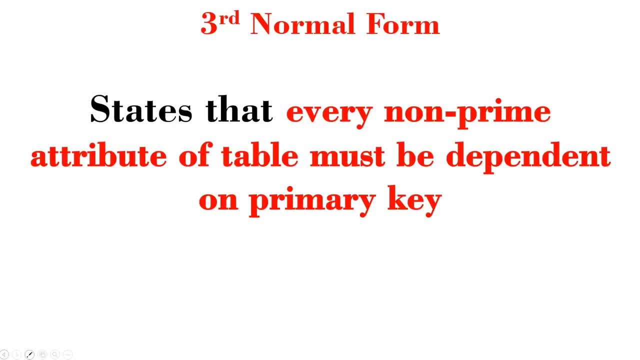 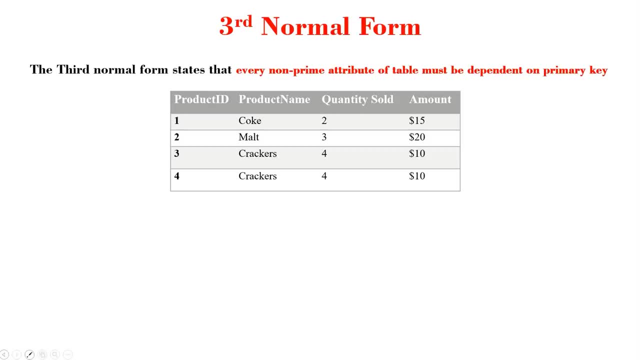 To explain this, I'm going to use the product table that we created under our second normal form. This is our product table that we generated under the second normal form. In this table, product name, quantity sold and amount are the non-prime attributes, and the rule states that all non-prime attributes 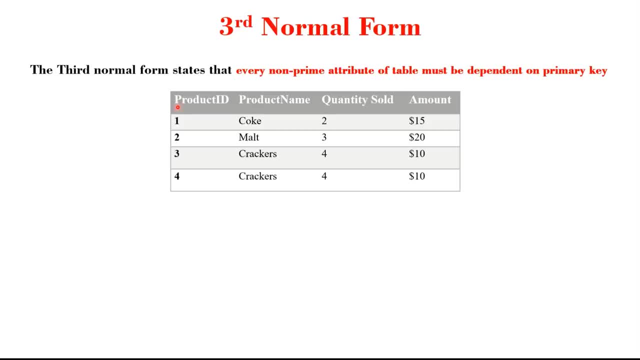 should depend on the primary key. It is true that product name, which is a non-prime attribute, depends on the product ID, the primary key. However, we cannot say the same for quantity sold and amount, as they are rather depending on the product name, which is a non-prime attribute, and this violates the third normal form. 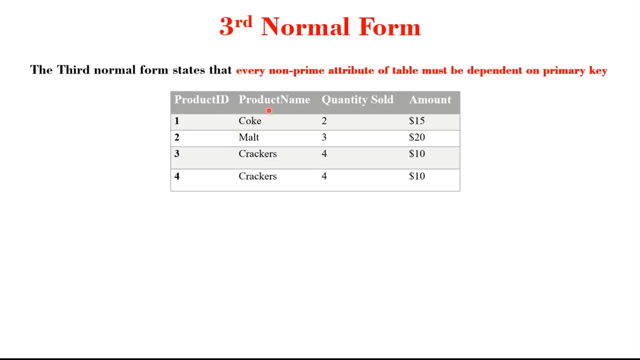 So for this table to satisfy the third normal form, again, we have to break the table down into new tables and provide primary keys for each of the tables, as you can see here. So now we have the product table and it is uniquely identified by the primary key, which is the product ID. We also 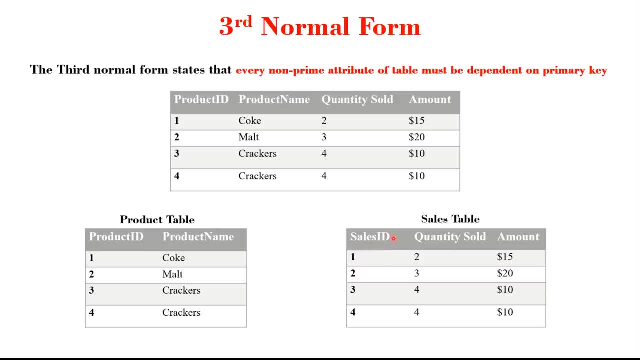 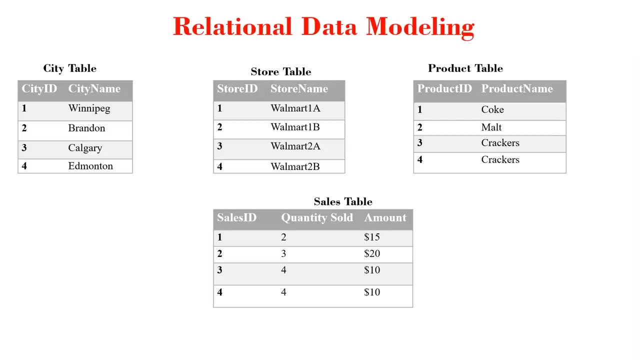 have sales table which is being uniquely identified by sales ID and the quantity sold and amount now fully depends on this sales ID primary key. So at this point we can say that our product sales table has been normalized to the third normal form. So far we have been able to normalize our big 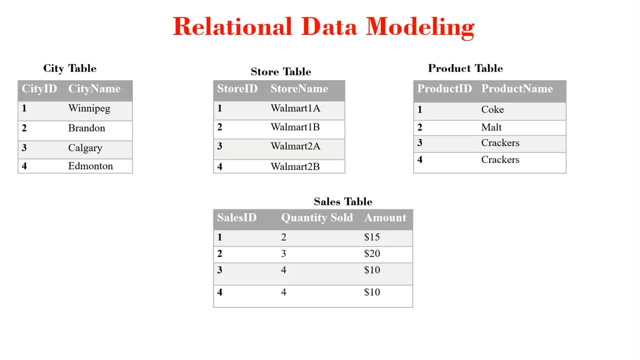 chunk of table into four tables. But remember, this is a relational database, so we have to show relationships between these tables and to do that, that's when my storytelling skills comes in. Think of it this way that you have a city and in each city you have store. So I'm going to link the city table to the store table as this, Also within each. 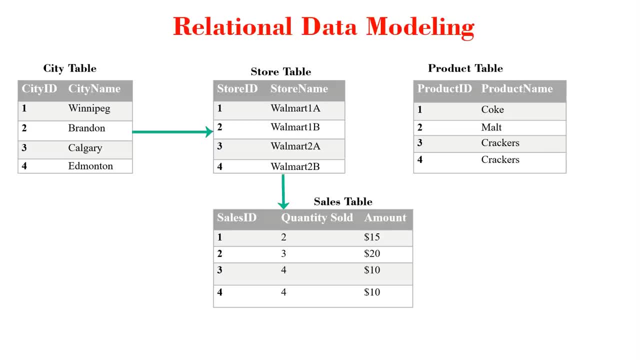 store sales are being made, so I will link the store table to the sales table. We also have product table, so we know that products are the items being sold, so it will make sense to link the product table to the sales table. So this is the relationship that you can generate for your normalized tables. The 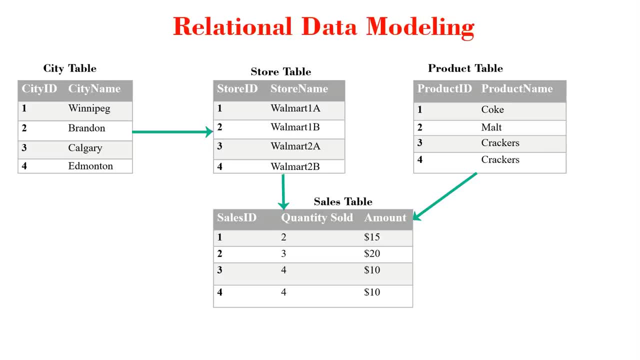 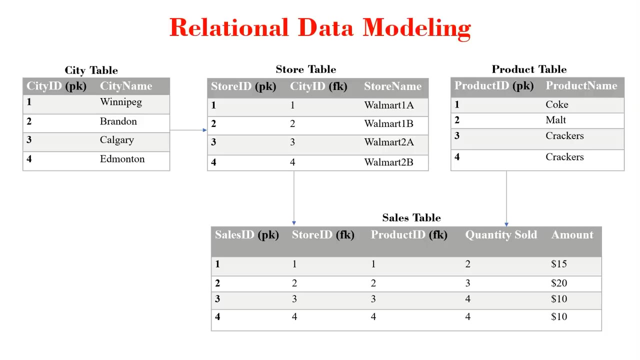 way to indicate that a table in a relational database is linked to another table is if you link them together using their unique columns. Oftentimes the primary key in table A will have to be listed in table B as a foreign key. So, for instance, in this city table I have city ID and. 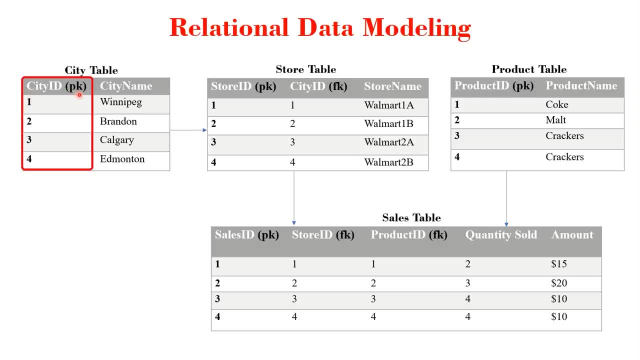 city name. City ID is the primary key. So in order to link this city table to the store table, I have to include the unique identifier of the city table, which is the city ID, in the store table as a foreign key. So this is a primary key in the city table will be included in the store table as a foreign. 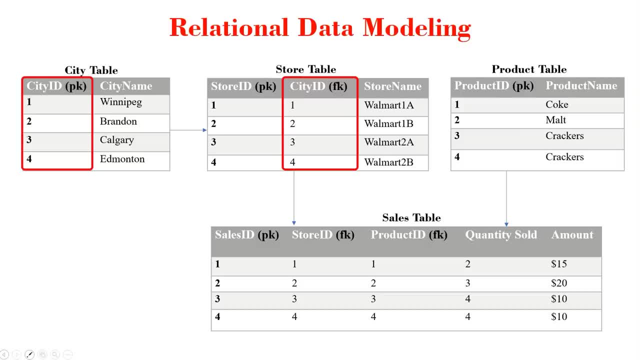 key. So this establishes the relationship between the two tables. Foreign key also ensures referential integrity between two tables, such that if data does not exist in the city table, the database management system will not permit you to enter that data in the store table, For instance. it is impossible to have this rule in our database management system. Why? Because we 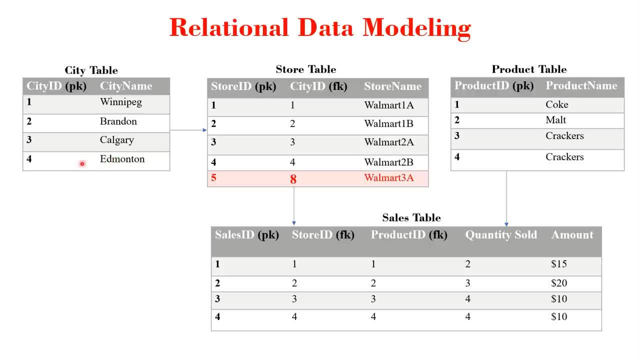 do not have any city ID 8 in the city table, So this is going to throw an error if you try to enter such data in the store table 8, as the city ID has to be listed first in the city table before it can be added to the store table, The only time you can be able. 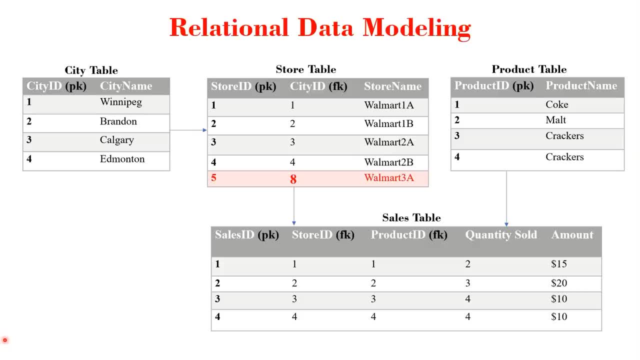 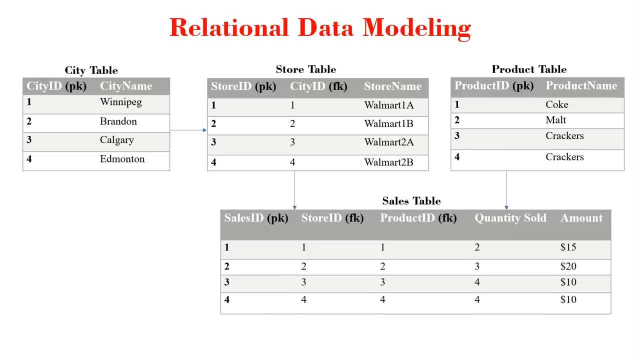 to do that is if there is no relationship between these two tables. But to ensure that accurate data is being installed in our database, it is always advisable to have a relationship between these two tables. So this should be our correct relational data model for the case study. 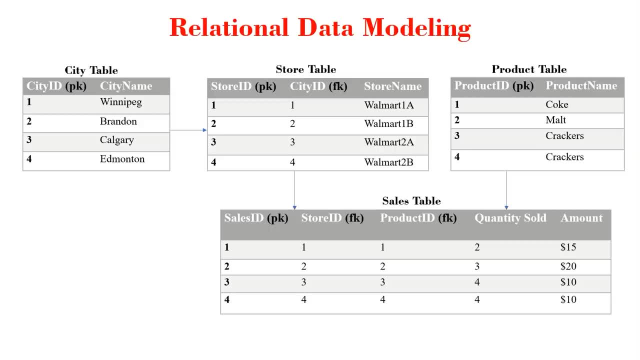 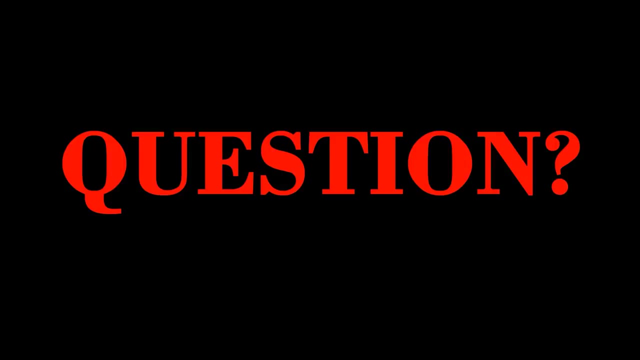 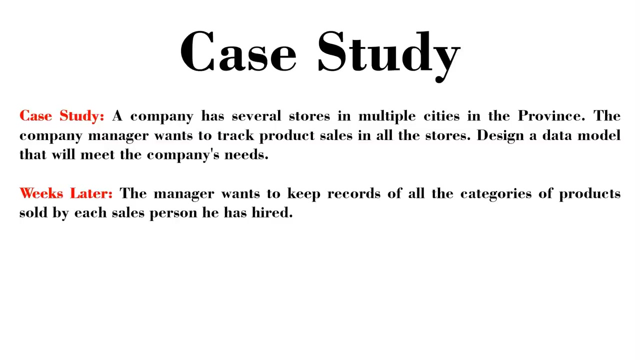 If you have been following our introduction to data modeling videos, you would know that up to this point, we have covered the conceptual models. At this point I have a question for you. If the manager now wants us to keep records of all categories of products sold by each salesperson, how? 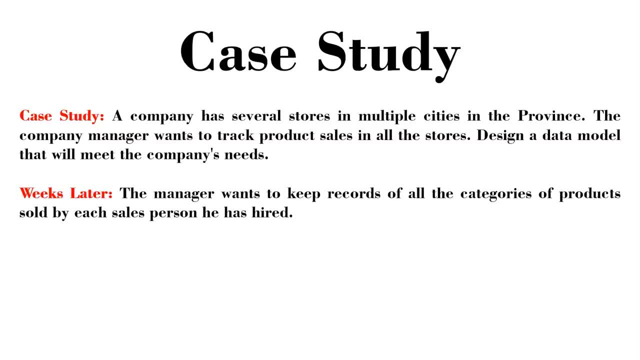 will our design look like? Remember, he now wants us to keep record of all product category, so that can be one table and also salesperson, So salesperson is also going to be another table. Okay, I guess you are done now If you answered. 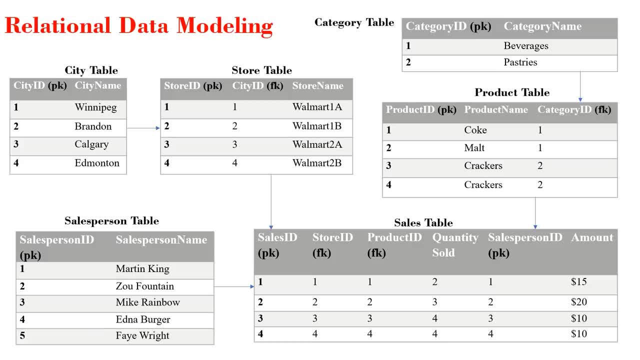 it correctly, then you should get a model that looks like this: Okay, Unlike the salesperson table, which links directly to the sales table, the product category links to the product table and then the product table to the sales table. You cannot link the product category table directly to the sales table because you 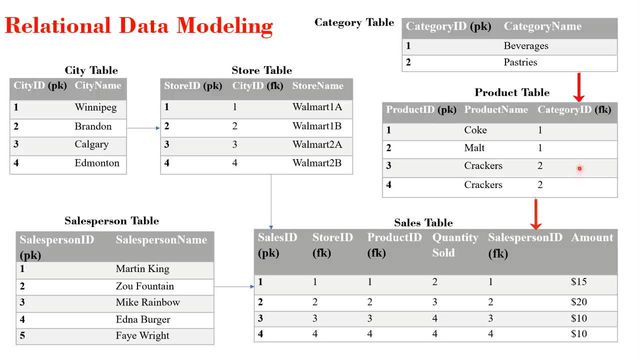 already have a product table, which is a subdivision of product category. So it's better to link the product category to the product table and then the product table goes to the sales table, More like a hierarchical form. This is: the highest level comes to the lowest.